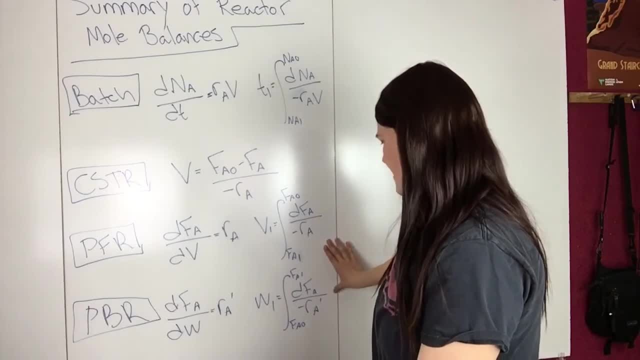 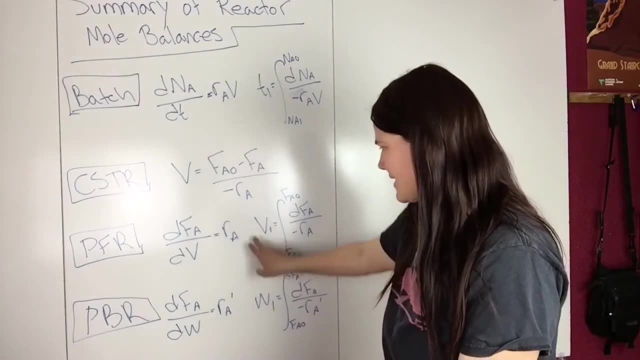 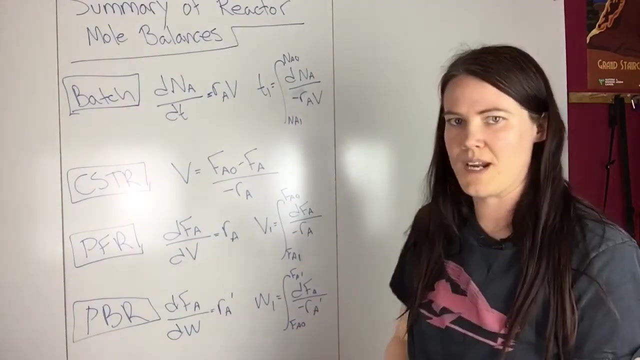 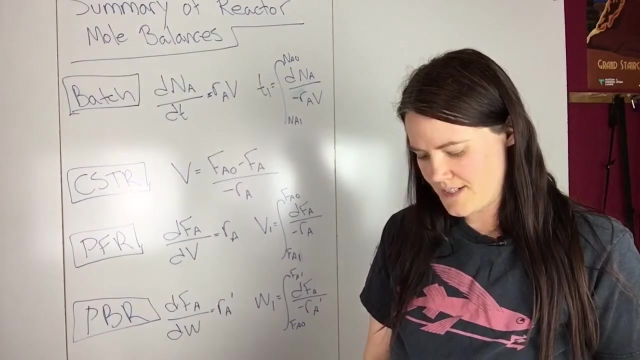 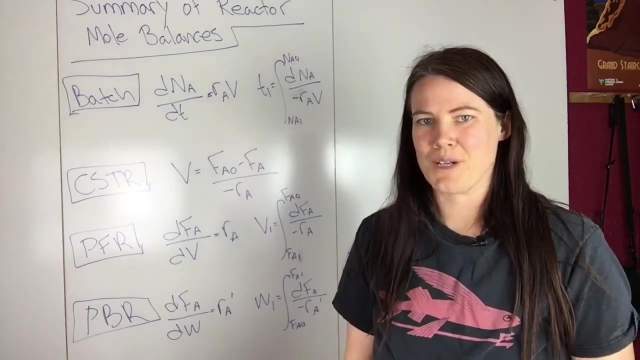 have the differential forms and the the integral forms, and these are really similar. the main difference is, for this one, you're calculating the volume of the reactor, and for the packed bed reactor, you're calculating the weight of the catalyst in the reactor. And so for this video I wanted to go over problem 1-15, so problem number 15- in chapter one of this. 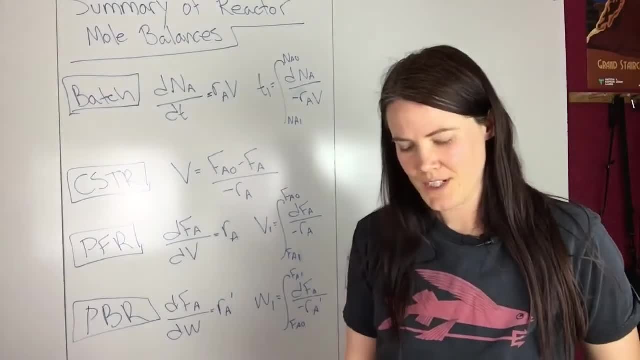 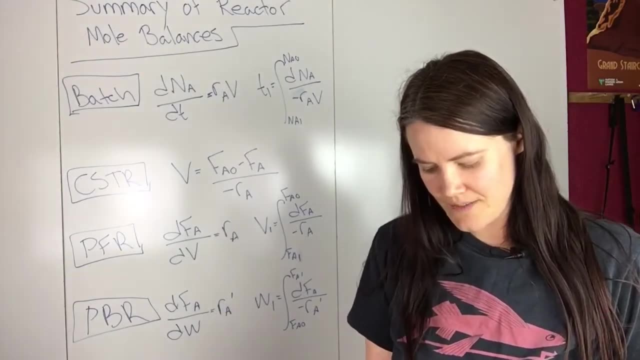 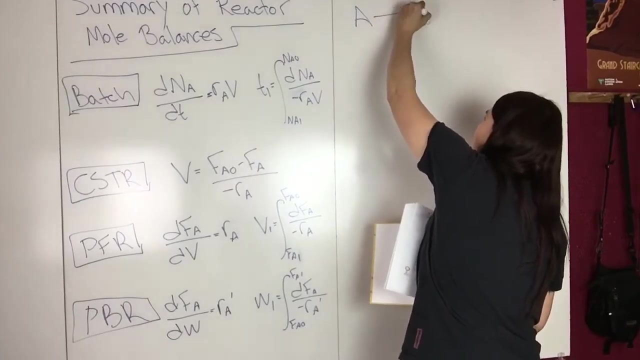 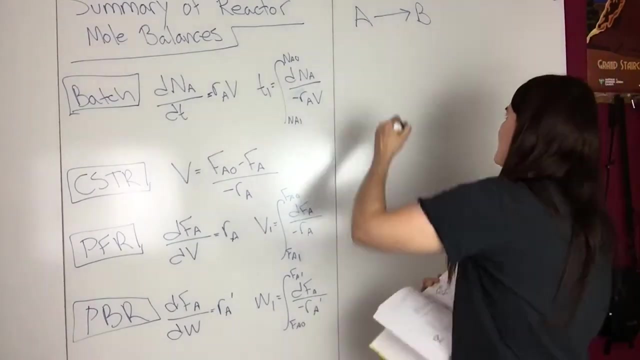 book the essentials of chemical reactor engineering by Fogler, and I have the four terms in the third and fourth edition. So this reaction is a to b. so you have, the reaction going from a to b is carried out isothermally in a continuous flow reactor. so first of all you can. 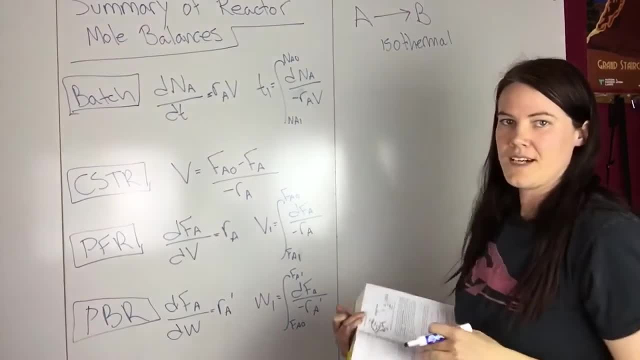 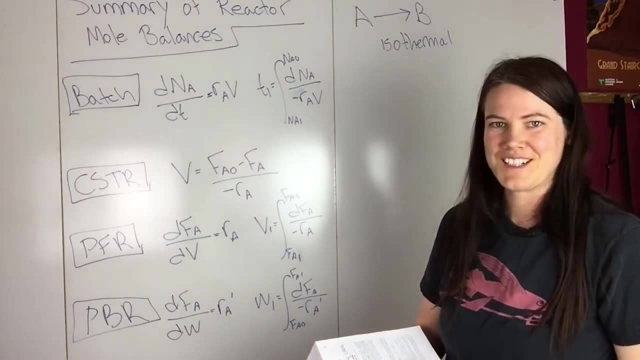 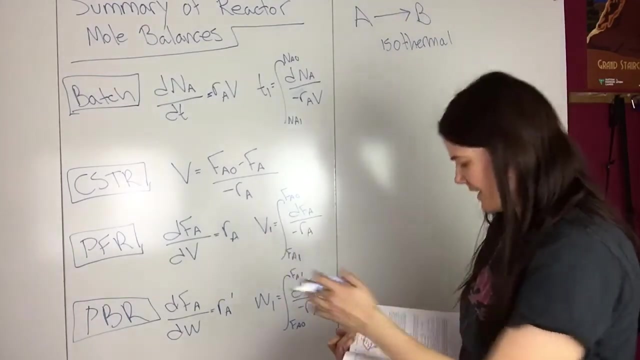 write down those isothermal, write down the information it gives you, because these problems can give you a ton of information and it can get confusing. So, anyways, continuous flow reactor, so basically a CSTR or a PFR or PBR, but it doesn't say: 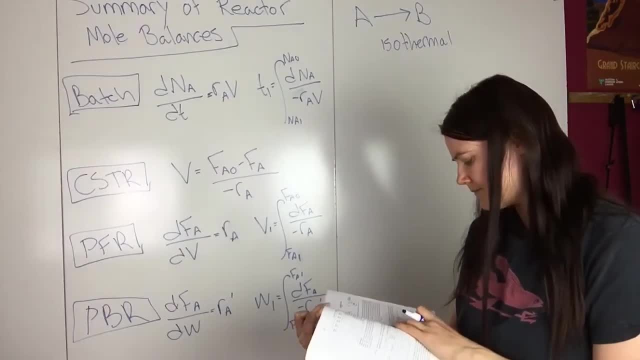 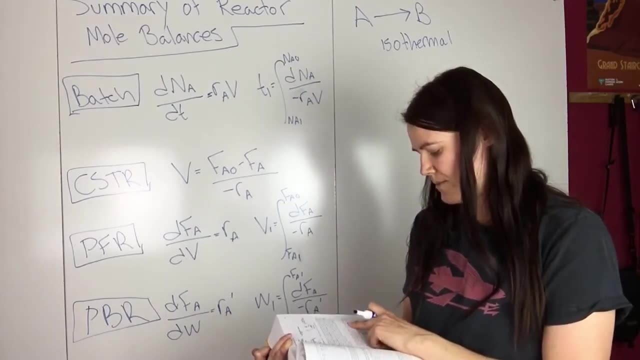 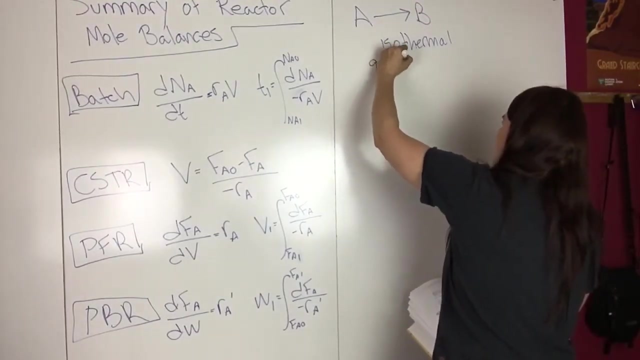 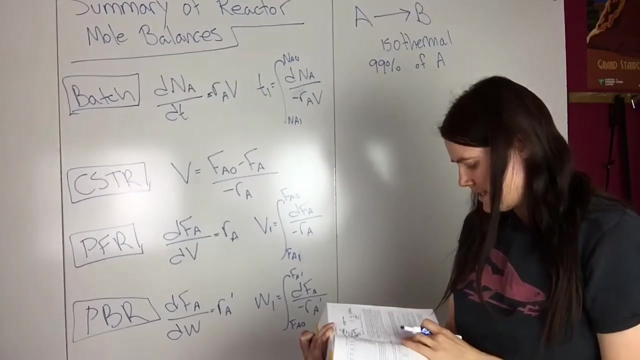 anything about this being a packed bed reactor. And then it says: calculate both the CSTR and PFR reactor volumes necessary to consume 99% of A. So we're consuming 99% of A and we're calculating the reactor volumes. 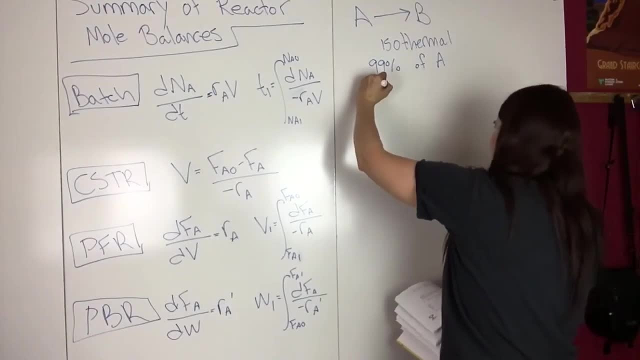 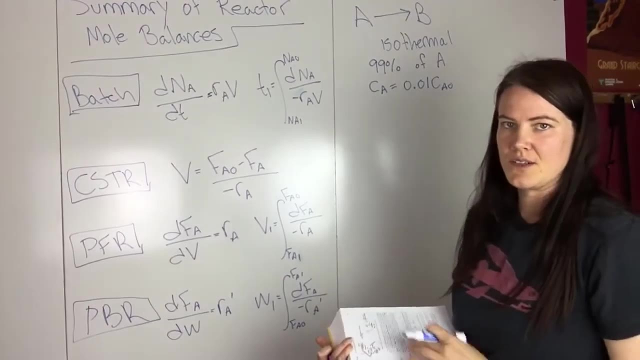 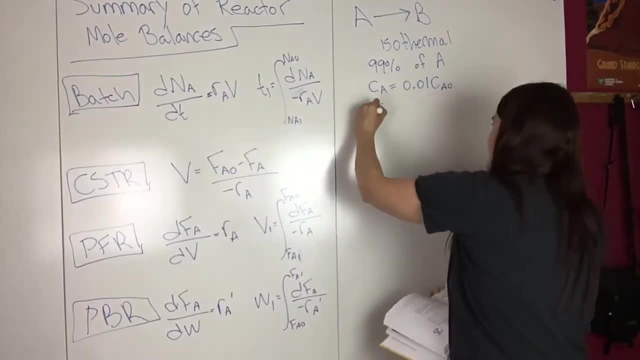 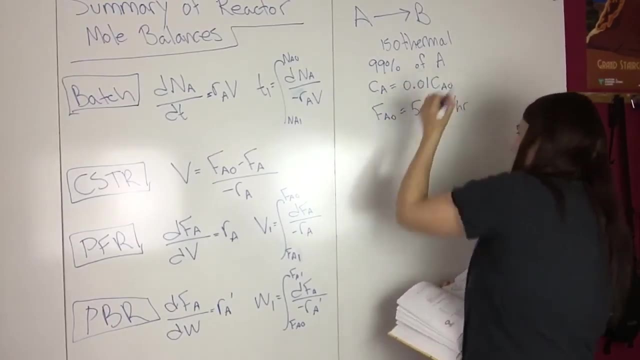 And we're going to go ahead and do that, And we're going to go ahead and do that, And we know that the entering molar flow rate, so FA-naught, is equal to 5 moles per hour. So we can write that down. 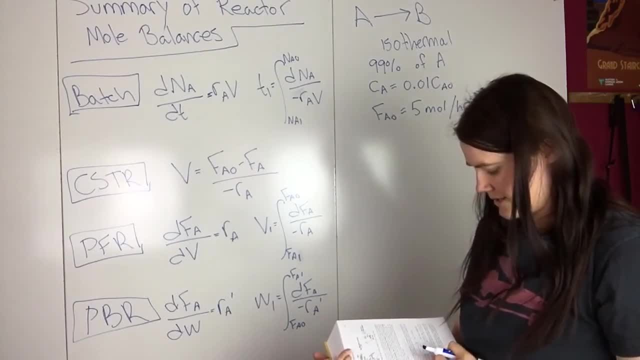 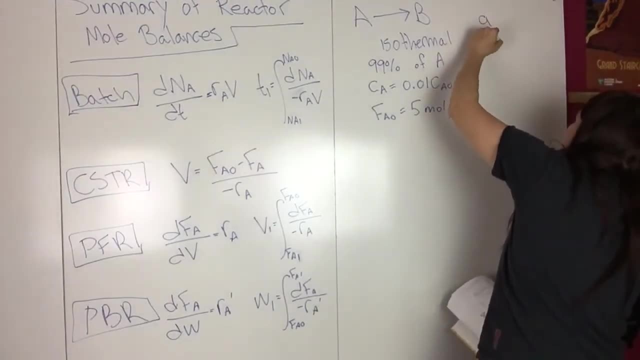 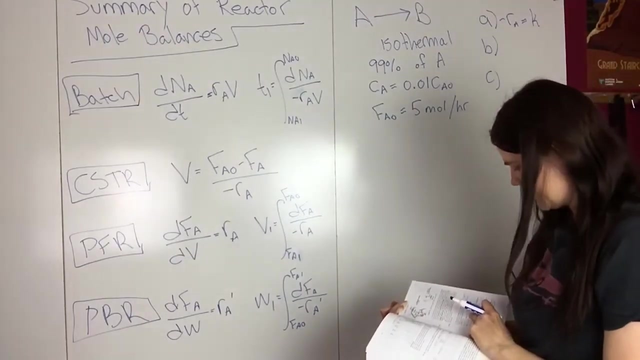 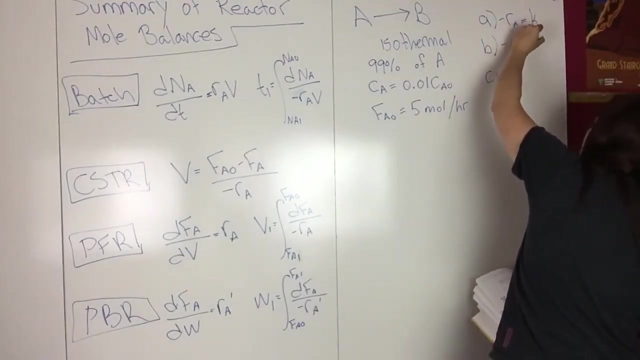 And then it gives you the equations for the reaction rates. So for A, B, C, So for A, It gives the rate as this, And then it gives you what K or what your constant is. And so for the next one, RA is equal to KCA. 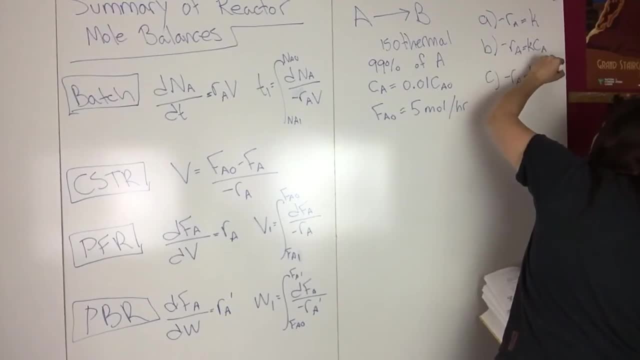 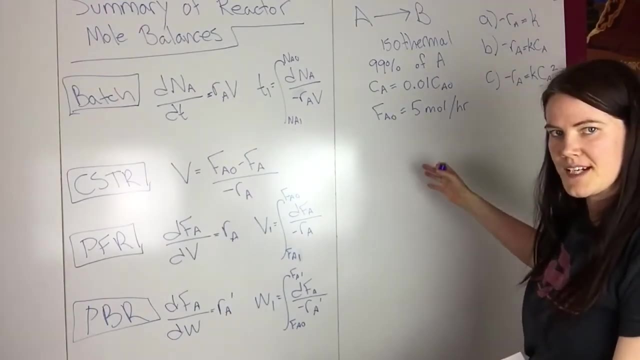 And then for the next one, RA is equal to KCA squared. So basically you're calculating The volumes for a CSTR and a PFR in each problem And you're just using different reaction rates. So this problem is really just plug and chug, once you get the right equation written down. 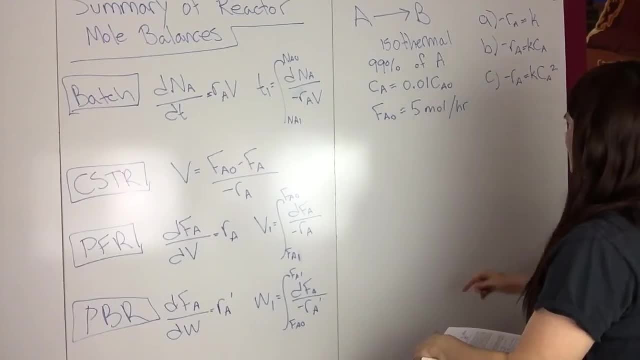 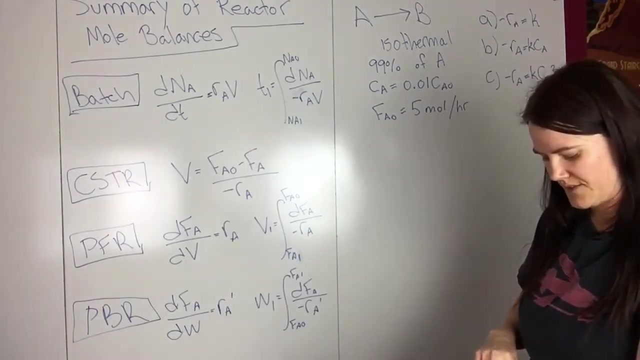 And so just one thing to notice with these reaction rates, So you can see that they- This one doesn't rely on concentration, These two rely on concentration, And this K is this constant which it gives you a number, A number of what it is in the problem. 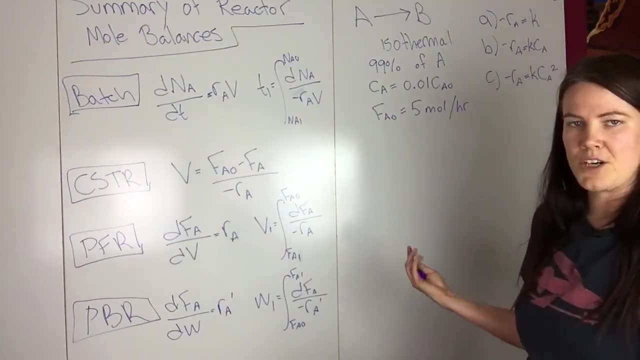 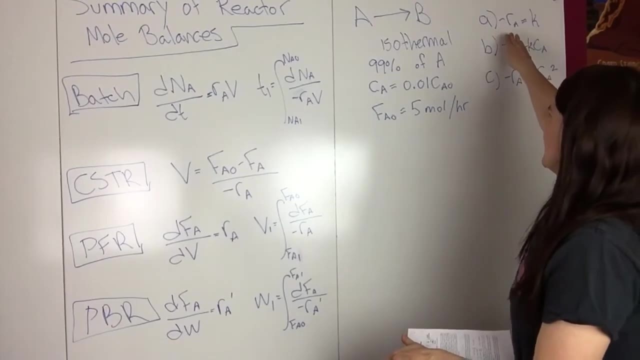 That constant is normally determined from experiments. And the other thing to notice is: the reason why you have a negative sign here is because this is the rate of disappearance of A. A is disappearing If you were writing this equation for B, so if you had, RB, equals whatever. 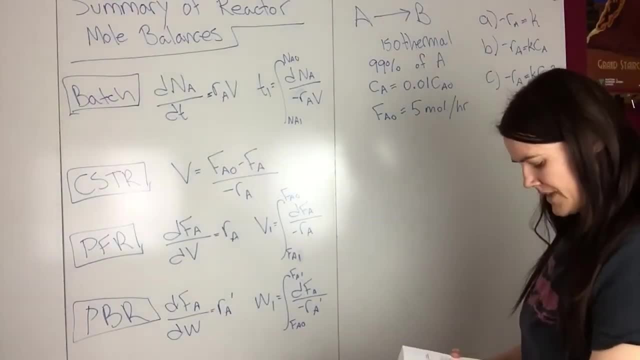 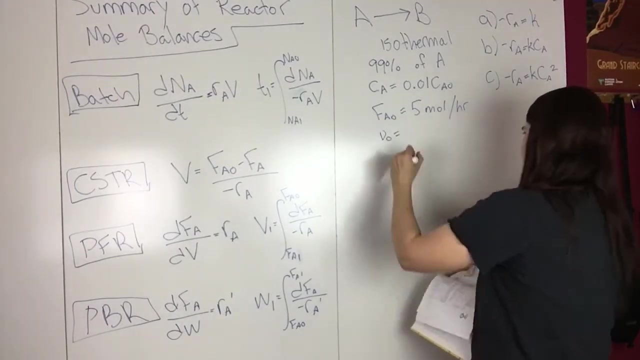 it would be positive because you're generating B, But because we're looking at A, it's negative, And so it also gives you the volumetric flow rate. So we know that the volumetric flow rate is equal to 10 dm cubed per hour. 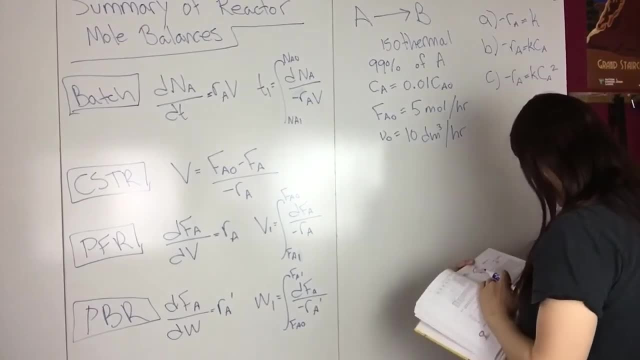 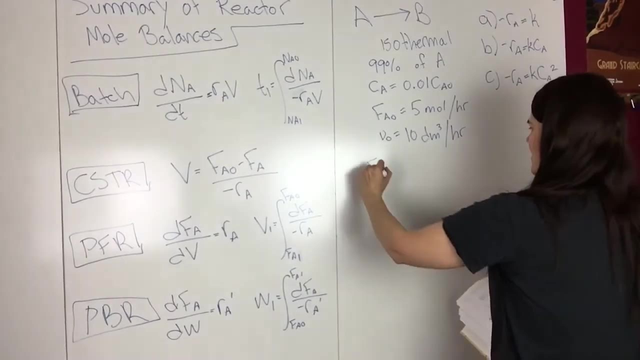 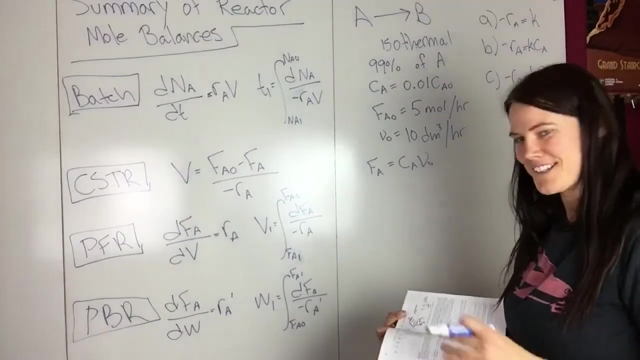 So it's a volume per time And it also tells you that your molar flow rate F A is equal to concentration multiplied by the volumetric flow rate. And this is a really useful equation to just basically memorize And Because you'll use it all the time. 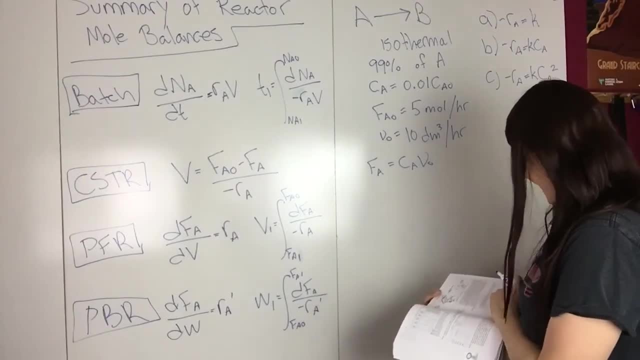 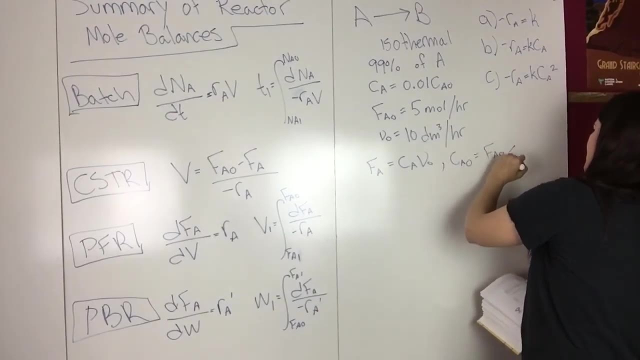 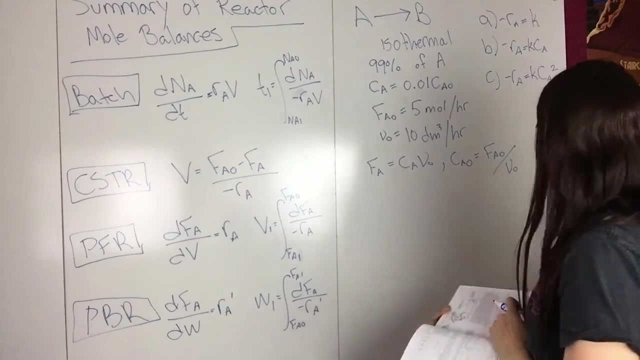 And let's see So. then, using that, we know that C A naught is equal to F A naught divided by B naught, And so from this, since it gives you these two things, you can calculate C A naught. 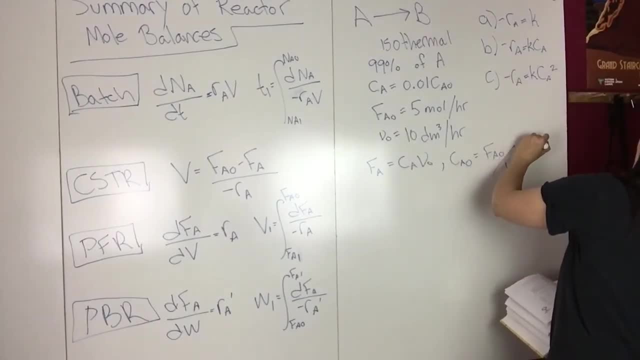 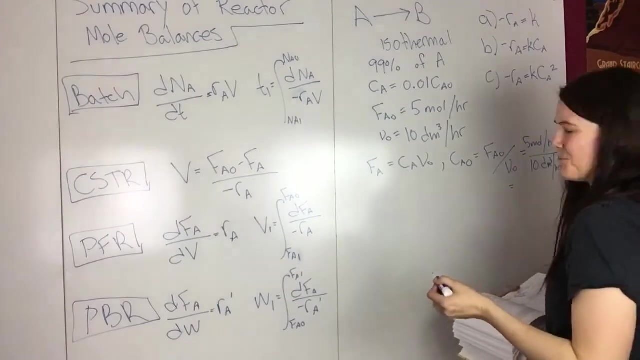 So we know that F A naught is 5 moles per hour And B naught is 10 dm cubed per hour. So then we end up with- And it gives you this in the problem, So then you end up with 0.5. 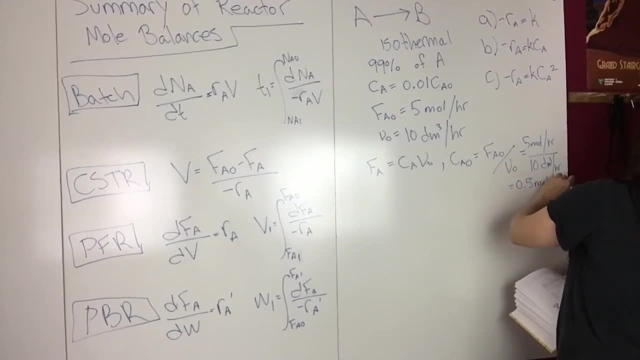 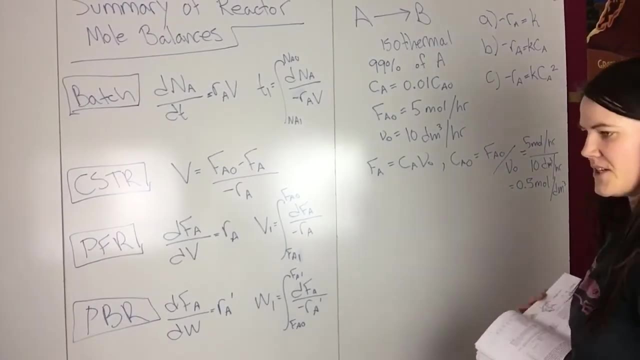 5 moles per dm cubed, And I always recommend writing down the units when you're doing these problems, because you, If your units don't work out the way they should, you know that you're doing something wrong And it 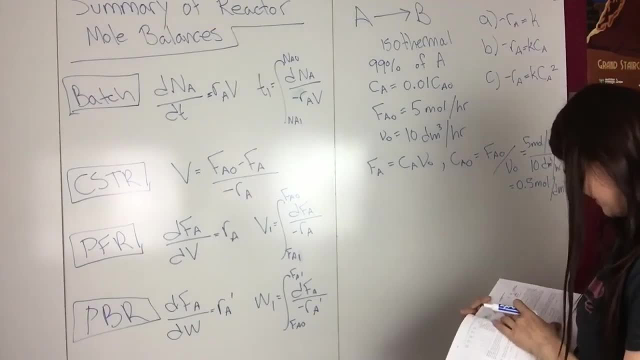 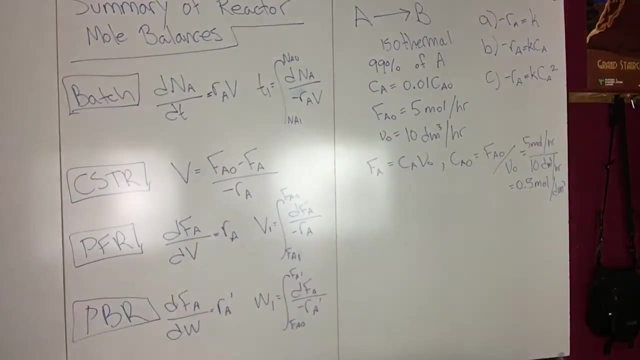 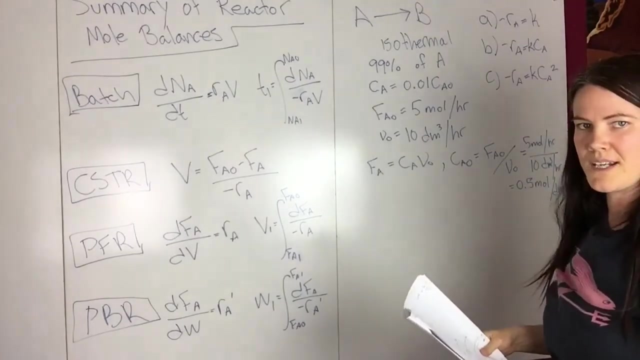 I think it just makes it easier, So It also gives you: Okay, so that's part D. Alright, so For part A or for A, first of all we want to calculate the volume of the CSTR necessary for 99% conversion of A. 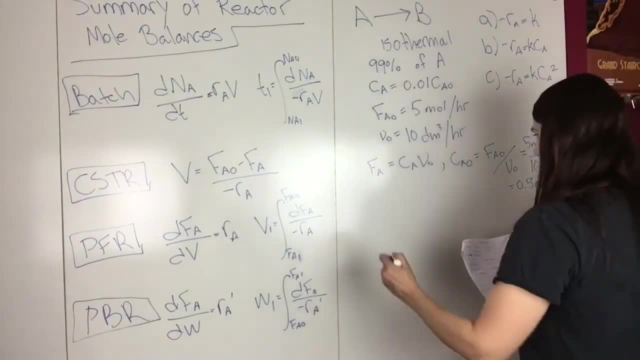 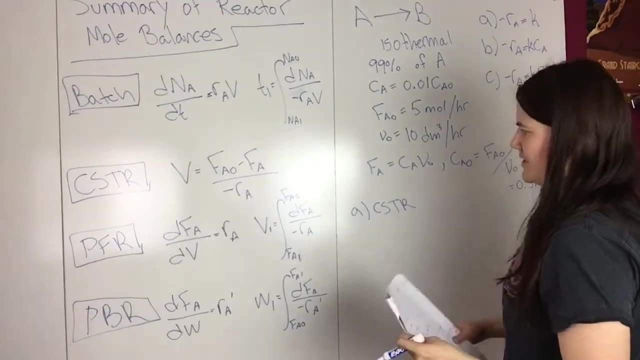 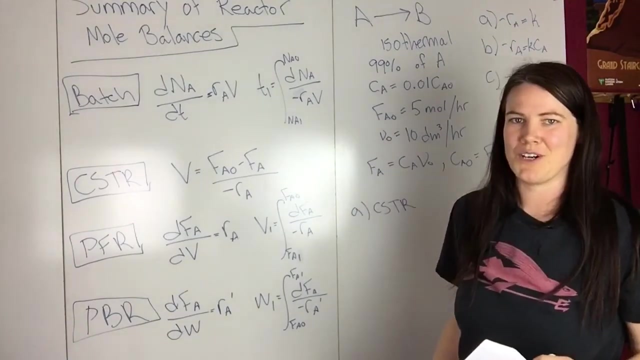 given all these parameters. So A For a CSTR. we can just go over here And these equations are summarized in Chapter 1.. And if you're curious where this equation came from, I derived it in the CSTR. It's in the mole balance video. so 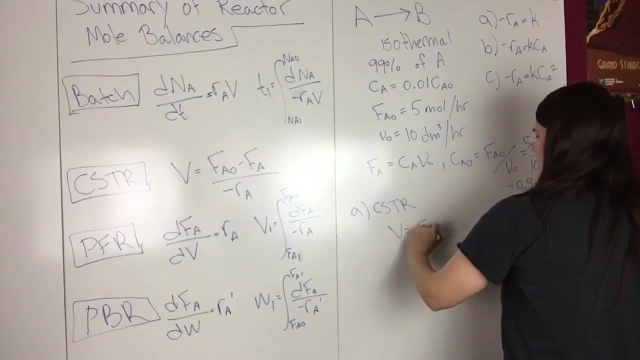 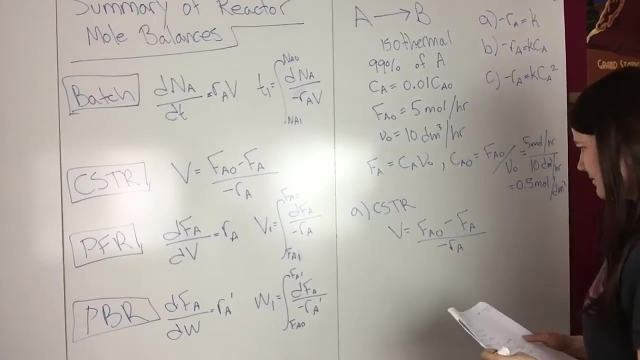 We can just write down this equation: V equals F A, naught minus F A over minus R A. How about It might be easier to solve this using the concentrations, so We can rewrite as, Since we know this, we can just plug that in. 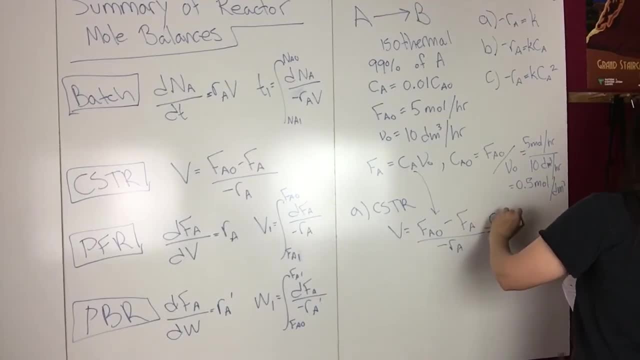 So then we get C A naught, B naught minus C A, B naught over minus R A. So then We know what all these are. So we know that We know C A naught. That's right here. 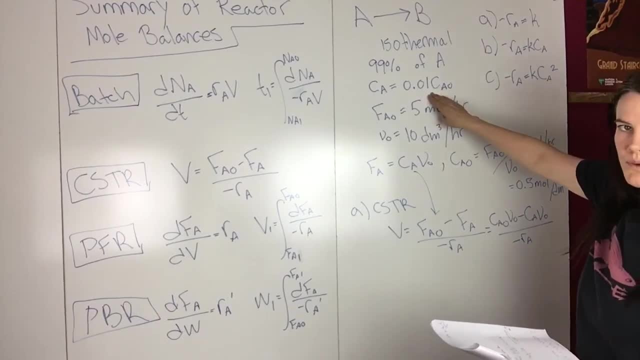 We know that C A equals point zero, one of C A naught. We know V naught the volumetric flow rate, And we know what R is- In this case it's just K- And So You would actually just do the exact same thing. 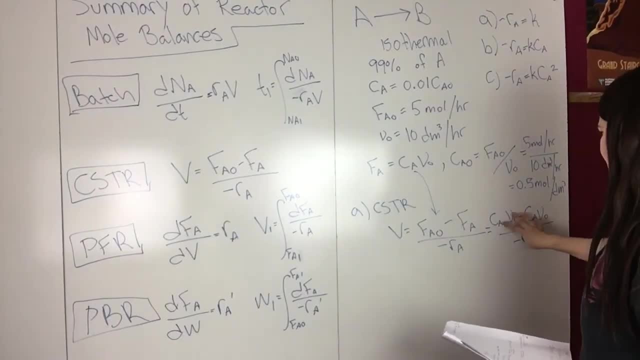 for A, B and C. So For B, it's all You plug in all the same. The only thing that's different is R, A. you know K and you know what C A is. So And the same thing for part C. 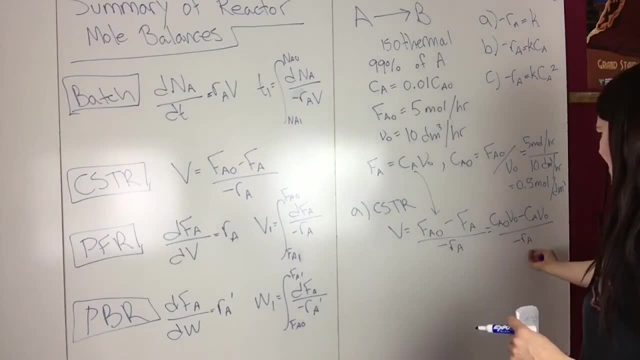 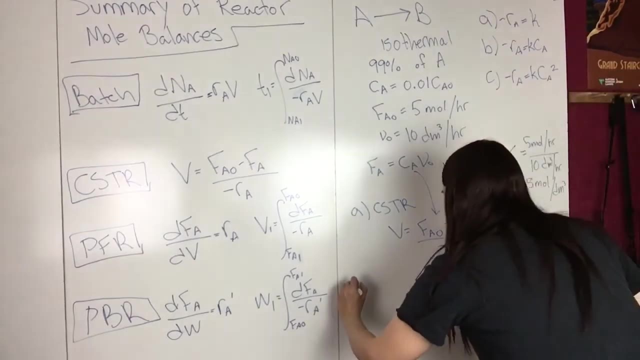 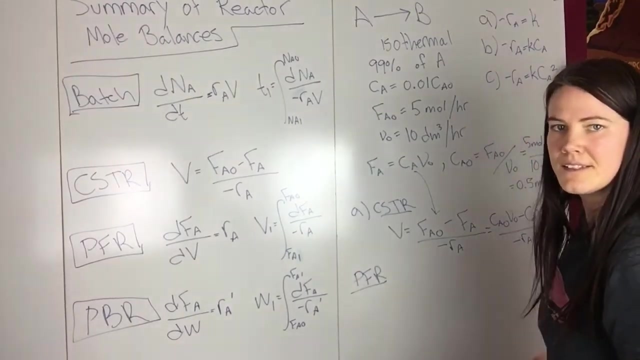 So That That problem is pretty much just plug and chug. once you get this equation And then For the P F R, so, And you can still see that, So for the P F R, we can go ahead and write down. 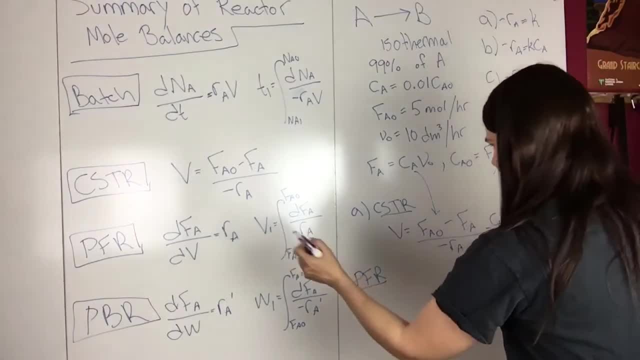 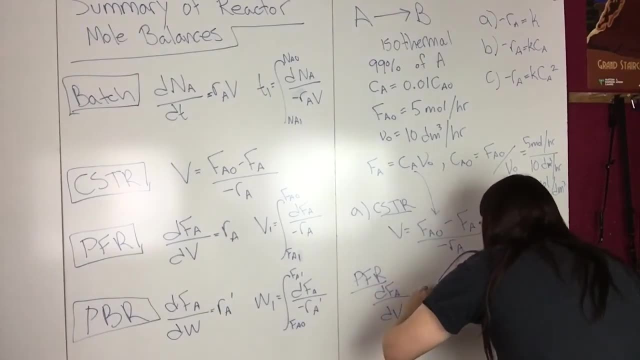 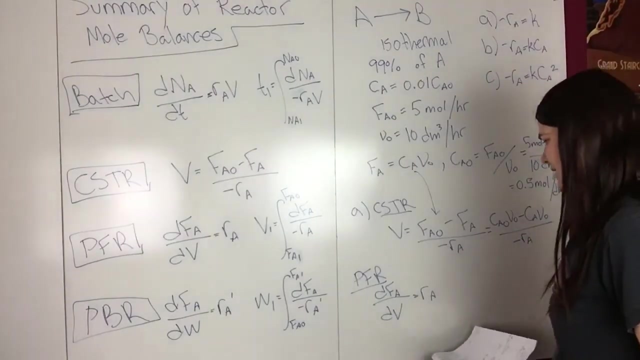 our equation. So D F, A over D V equals R A. And that just came from the summary in chapter one. And if you're curious how that's derived, I derived that in the video on the mole balance for a, P, F, R. 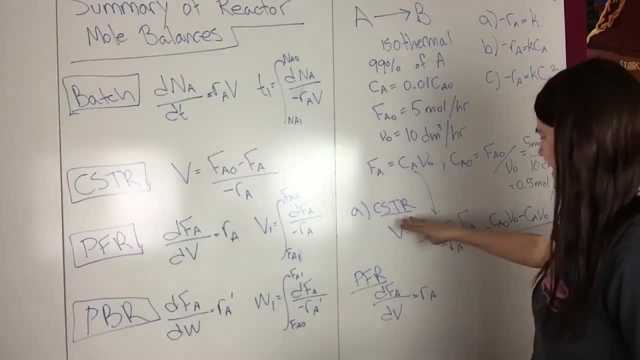 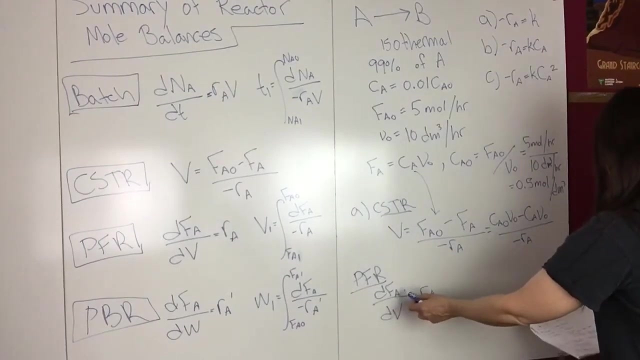 So then for part A. so The C S T R is pretty much the same for all the parts, but this equation will change slightly depending on what your, what you integrate. So If we go ahead and plug some stuff in, first of all, we know that F A 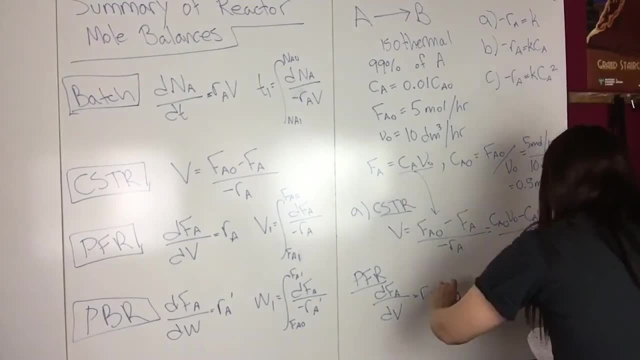 is equal to this. So We know that. We know that C- Well, D, C, A, B naught over D, B equals. And then R, A, that equals negative K, And the reason why this is negative is because that's. 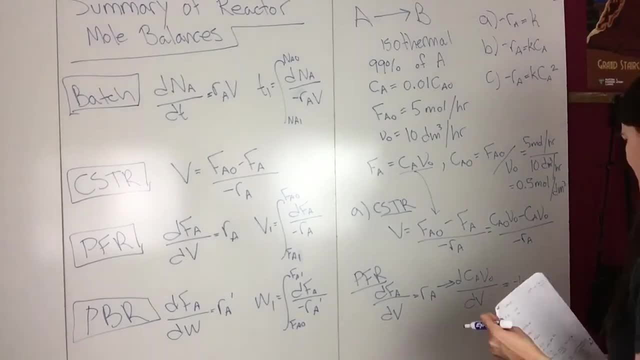 The R A is actually negative in this case, because we're looking at the disappearance and As opposed to the generation. So then, Let's see- I think you can still see this- So then, if we rearrange this, you get B naught. 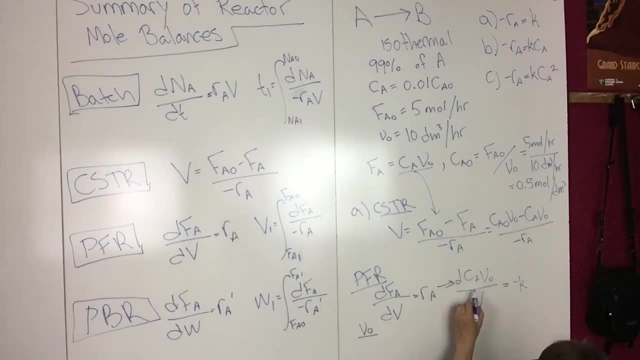 So We can pull B naught out, So we get. So pulling B naught out and dividing by K, We get C. And we want to integrate from C A naught to C A, D. C A equals zero, to V, D, V. 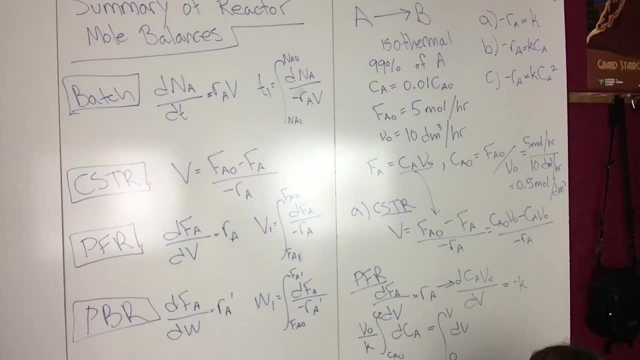 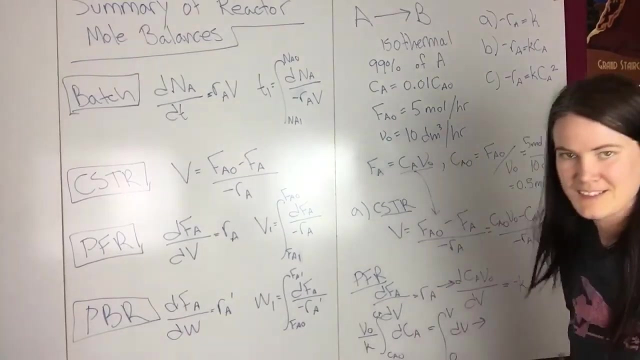 And then for the D, C A, the limits are just from the C A naught to the C to the, The initial concentration to the final concentration. So that's C A naught to C A, And so then, Yeah, you can still see that. 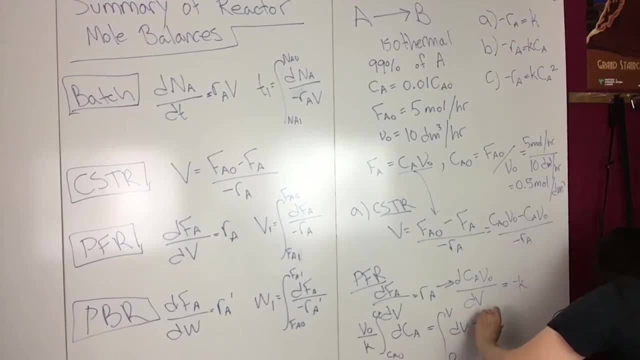 So then, taking this, Integrating this, we end up with V equals V naught over K, C A naught minus C A. And then we Should, We know everything for this, We know the volumetric flow rate, We know K because it's given. 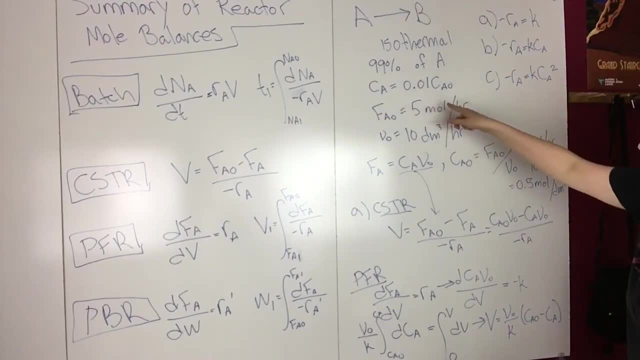 We know C A, naught, And we know C A, So then you can just plug everything in and solve that equation. So I want to erase some things, because the, The, The P, F, R for part B and C is slightly different, because 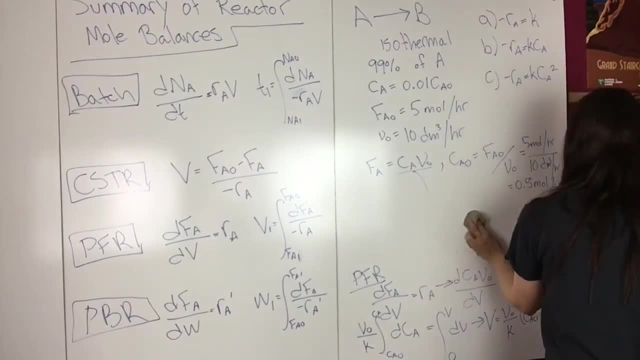 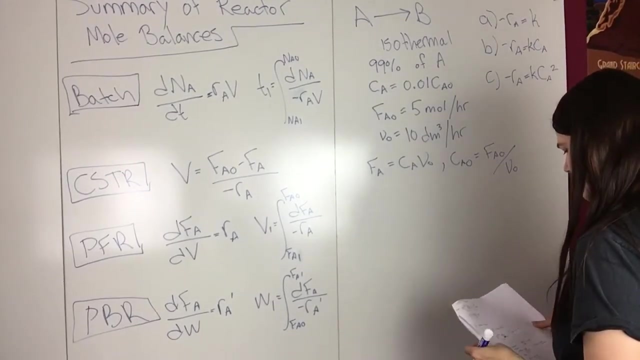 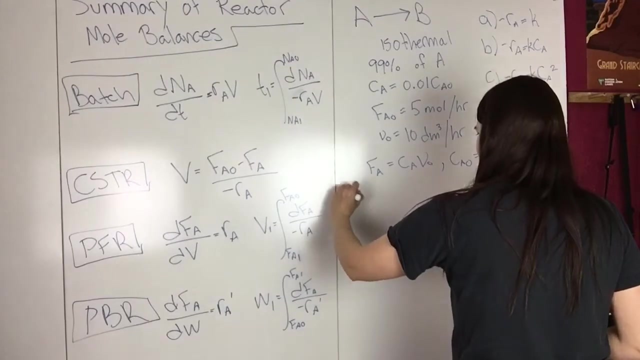 of your integration. So I'll just erase this real quick. All right, So for part B, once again we can write down the equation for a, P, F, R, which is So I'm doing B now. So this is D, F, A. 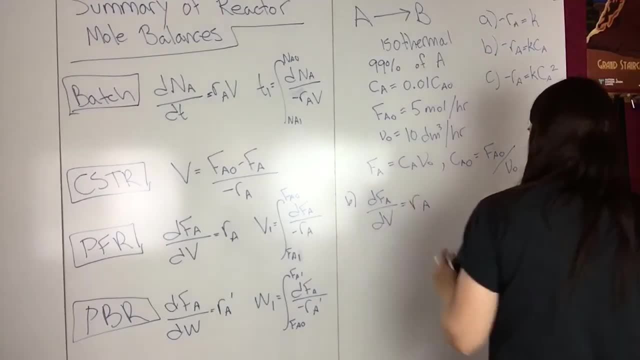 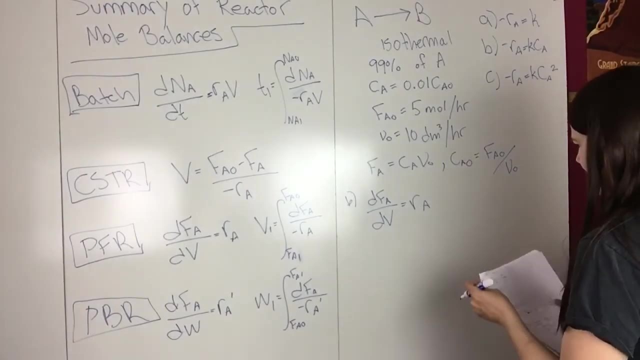 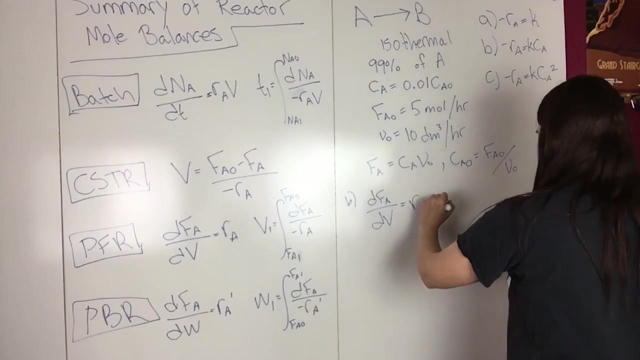 D, V equals R, A, And So then we can go ahead and plug in some of the information. So we know that D, Oh, D, F, A. So this is D, C, A, B, naught Oops, And that's from. 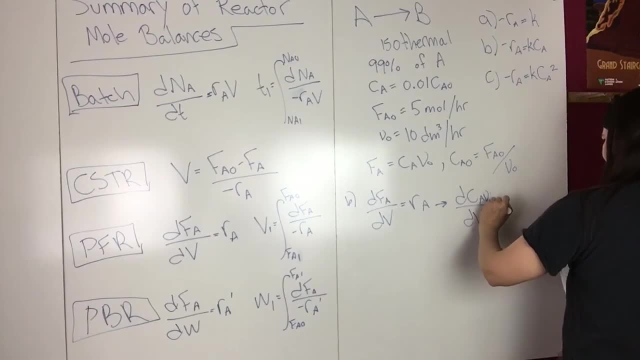 this equation: D, V equals, And then R A for part B is minus K, C, A, And so then we can go ahead and rearrange this and integrate. So first of all you can- Oh, I'll just write it down- 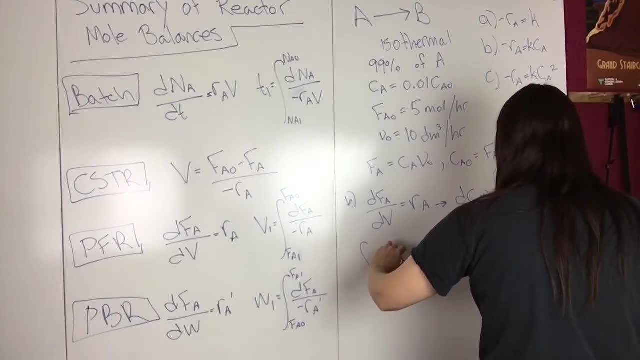 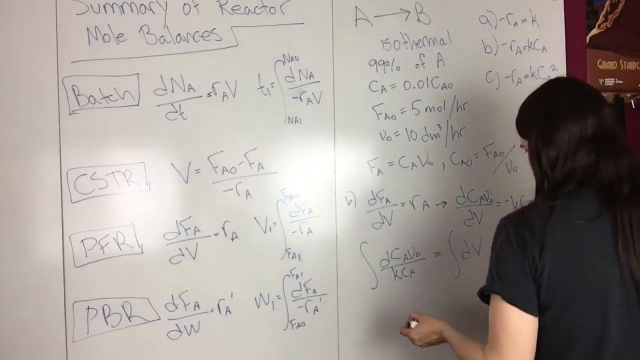 So D, C, A, V naught over K, C A equals D, V And First of all, we can pull the V naught and K out of the integral because they're cons. Yeah, they don't change so. 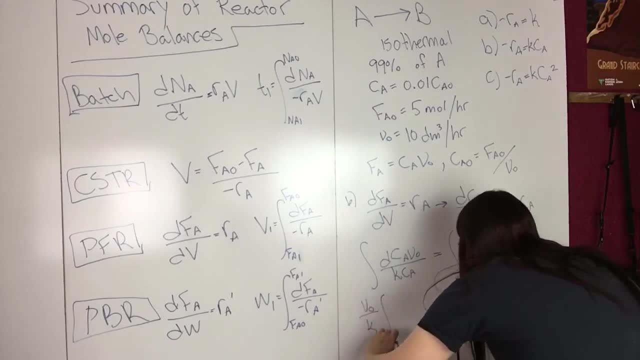 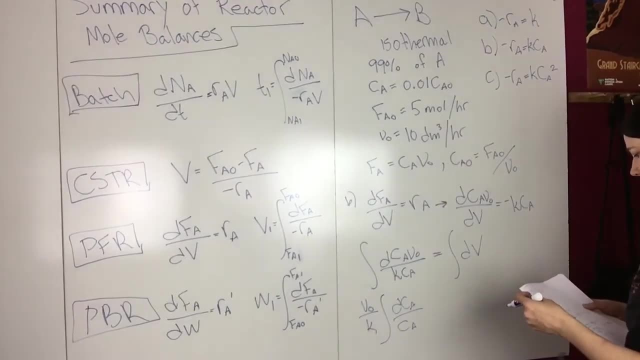 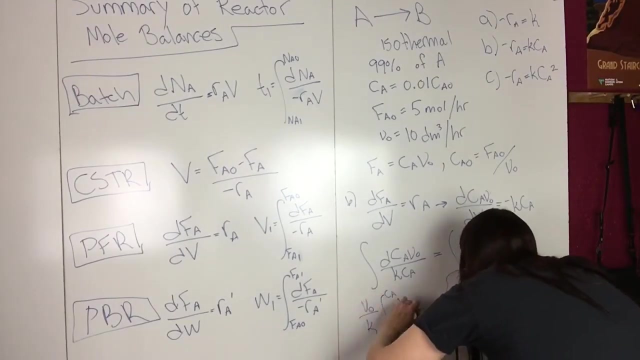 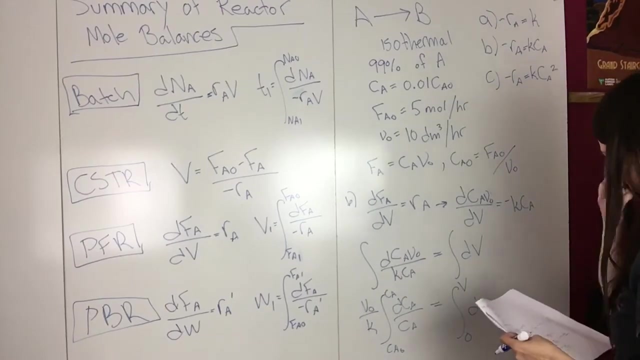 We have V naught over K And then. So then we have D C A over C A And we want to integrate from C A naught to C A, And then this one, we're integrating from 0 to V. So then, 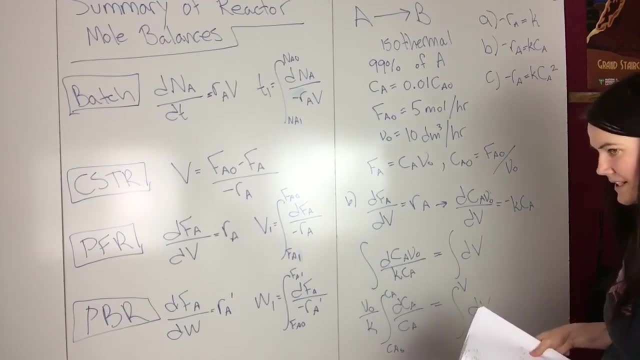 taking the integral of this, we just end up with basically V, And then, taking the integral of this, we end up with the natural log of C A naught over C A, And if you can't remember how to do that, then just Google it. 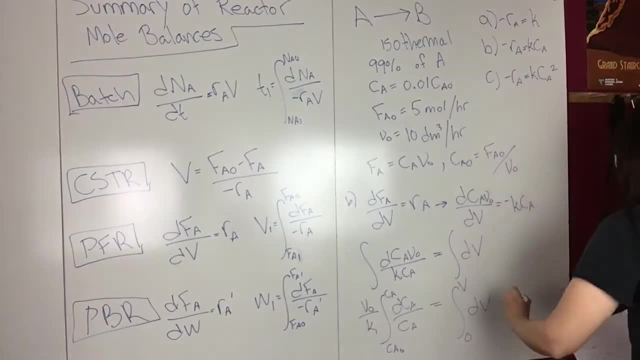 or look at Wolfram Alpha, And So anyway, we end up with V naught over K, natural log C, A naught over C. A equals V, And then we're solving for V and we know everything else. So We know C A naught. 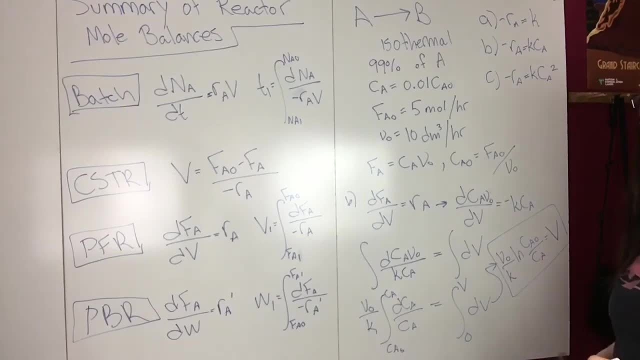 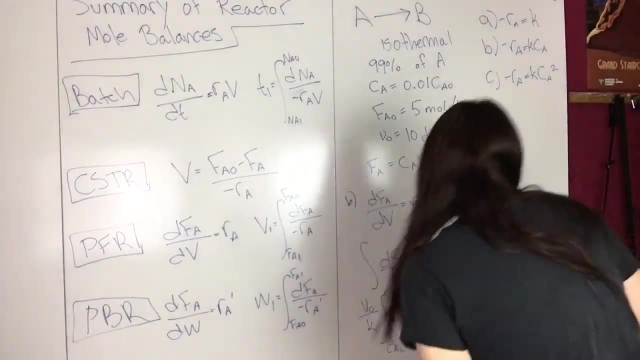 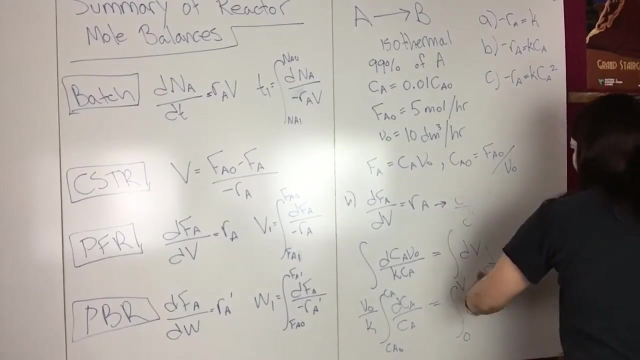 We know C, A, We know V- naught, And we know K. So at this point you can just plug everything in and solve it, And then for part C, it is pretty much the. You start with the same equation, The only. 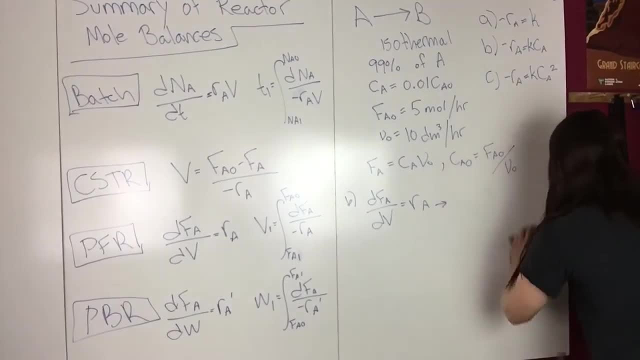 difference is you have. Well then, for part C, the CSTR is still the same. This one changes because of your integral, Because, instead of for R, Well, I'll just write this down again: So R A. So then plugging things in. 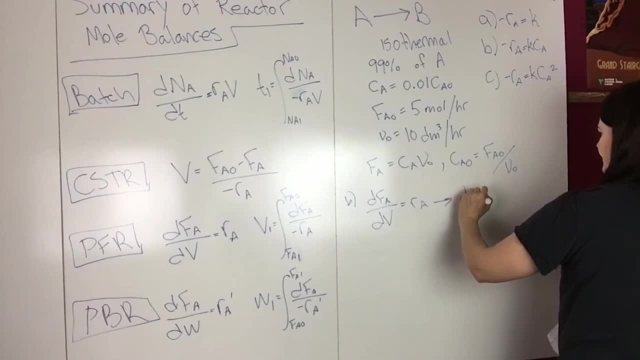 for this one you have the D C A V naught over D V equals. And then for part C, R A was K C A squared. So you can see that when we rearrange and integrate this, this is going to be. 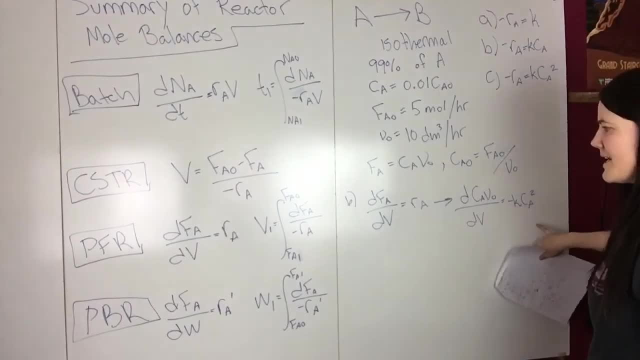 integrated slightly differently from how it was in A and B, Because you have C A squared instead of C A or just the K. So rearranging this we have. Let's see. Well, same thing. So divide the K and. 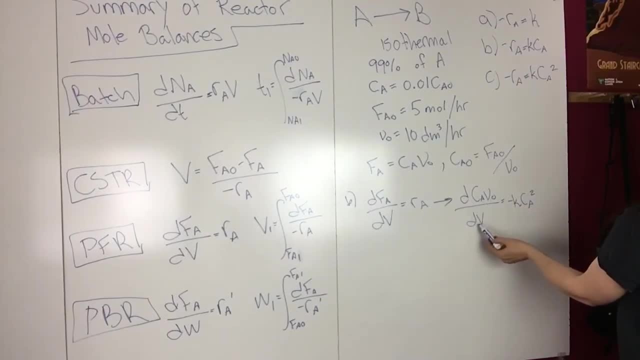 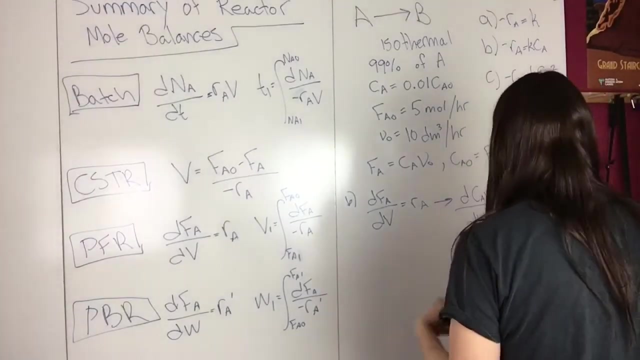 C, A squared over, And divide Or multiply the D, V through, And then you can pull the V, naught and K out of the integral, Because they don't, They're not dependent on, So they're basically constant. So. 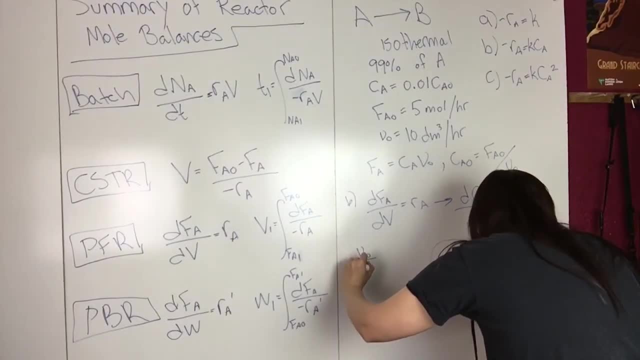 With that. So then, with that, you get V naught over K, And once again we're integrating from C A naught to C A D C. This is D C A over, So D C A over C A, squared equals. 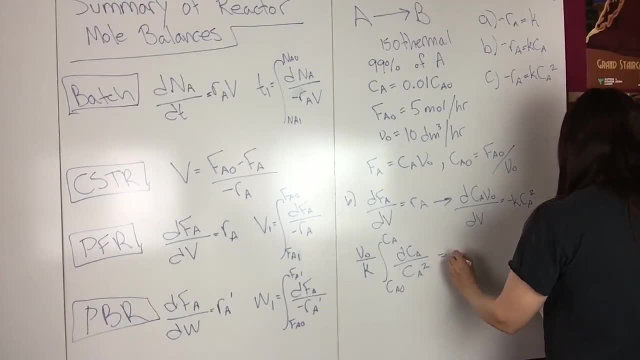 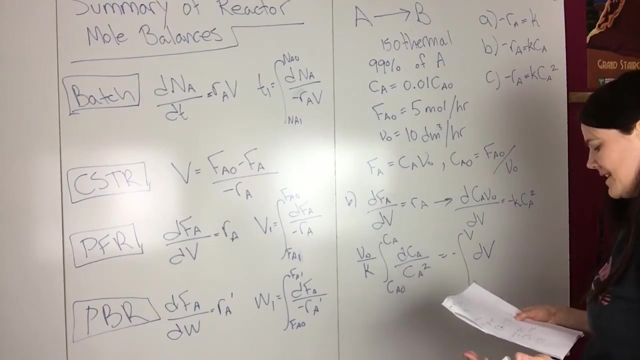 and then this is zero to V D, V, And so then, integrating this, you're going to end up with the one over C A minus one over C A naught. And once again, if you don't remember this integration, then just look it up on Google, or. 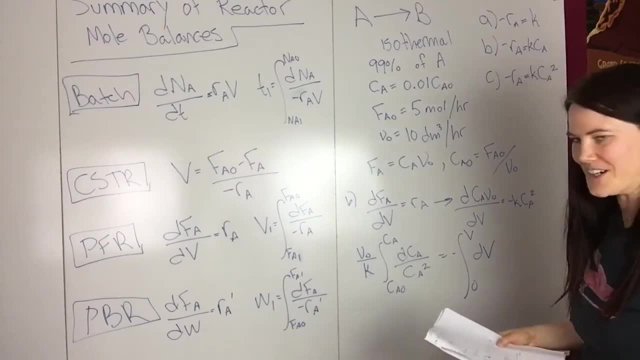 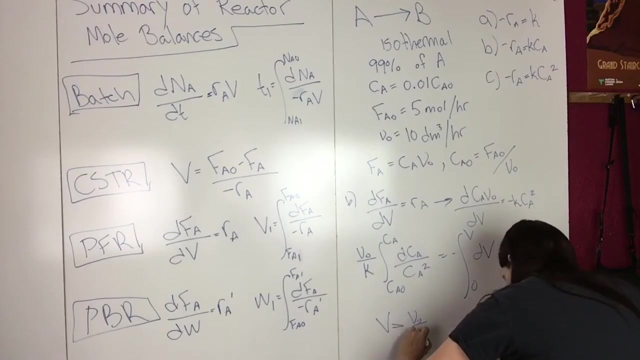 Wolfram Alpha or your calculator, And So, anyway, integrating this, and then this is just: When you integrate this, you just get V, Or you just get the volume. So V equals V naught over K, one over C A. 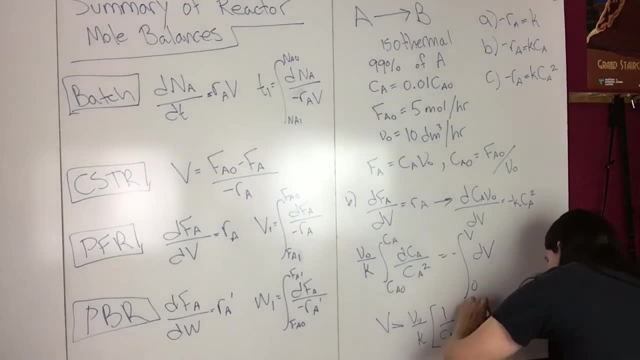 minus one over C A naught. And so then you should just be able to plug everything in and solve that, because we know V naught, We know K, We know C A And we know C A naught. So then, for part D, it tells you that 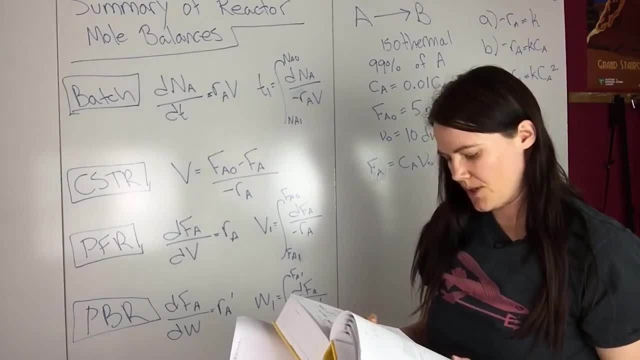 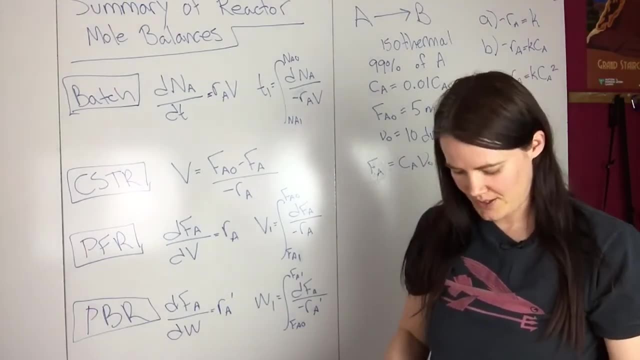 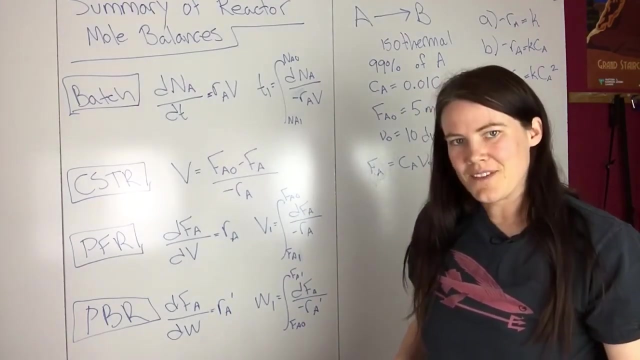 to repeat A, B and C for a batch reactor. So this time we're calculating the time required for the reaction instead of the volume of the reactor, since it's a batch reactor, And So it's kind of the same thing, only we're using a different. 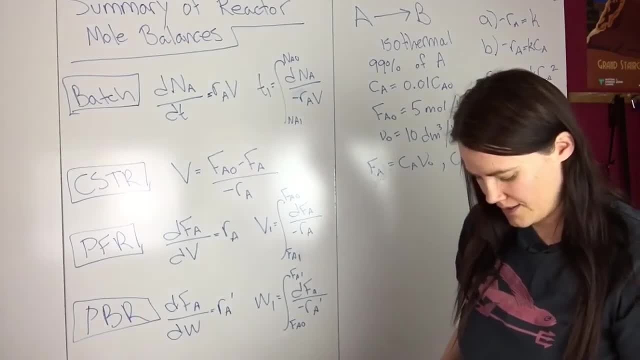 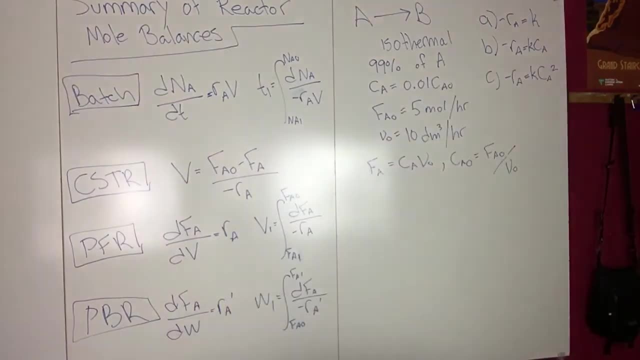 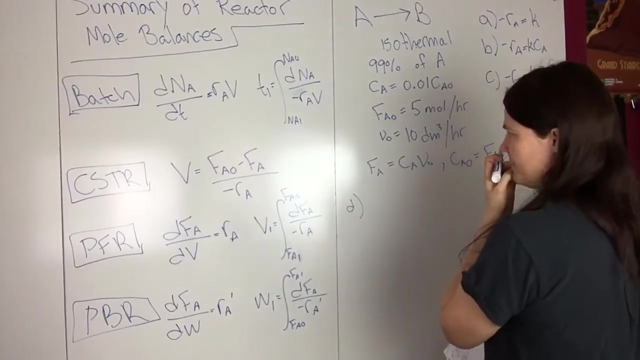 mole balance, because we're using a different reactor. And then You, And then you're plugging in the Like, So you're calculating it for each of the reaction rates. So For Part D, First of all I'll write down the 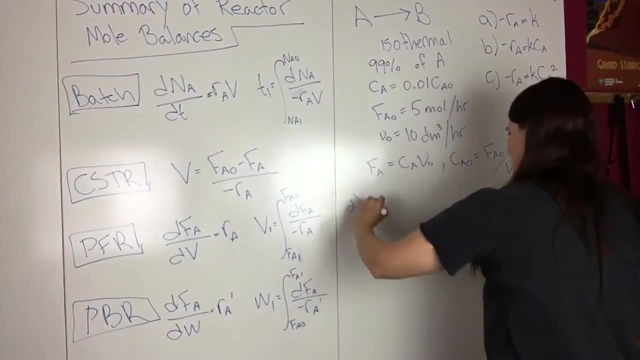 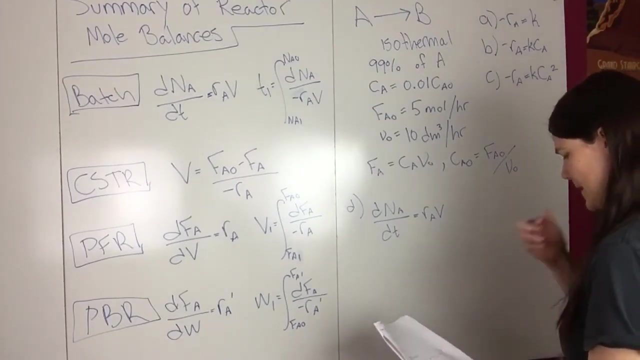 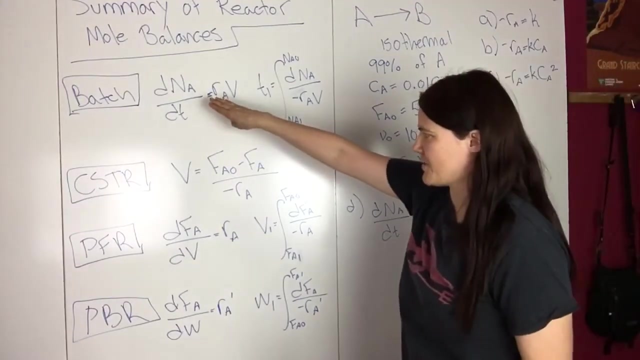 differential equation for a batch reactor. So D N A over D T equals R, A, V, And. And One thing you might notice with this is this: A batch reactor is written with a change in moles instead of a change in the. 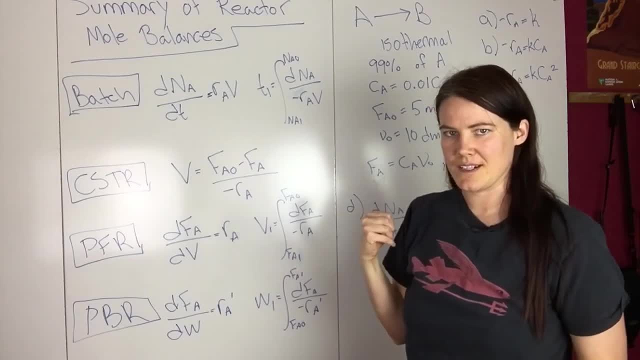 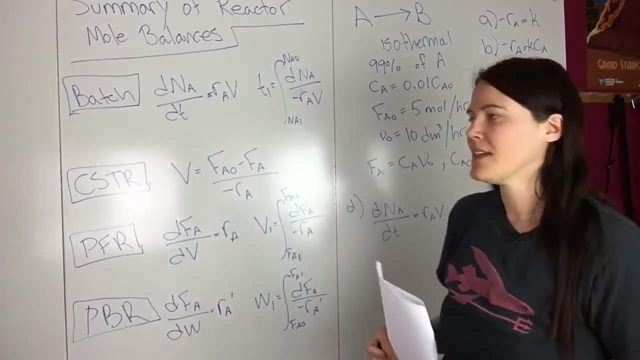 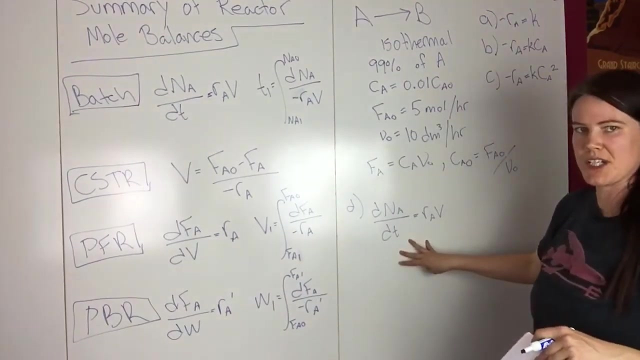 In the Molar flow rate, And The reason why is because in a batch reactor you don't have flow, You just have something sitting there, So that's Why that's written differently. This, The method to solve this one, is pretty much the same. 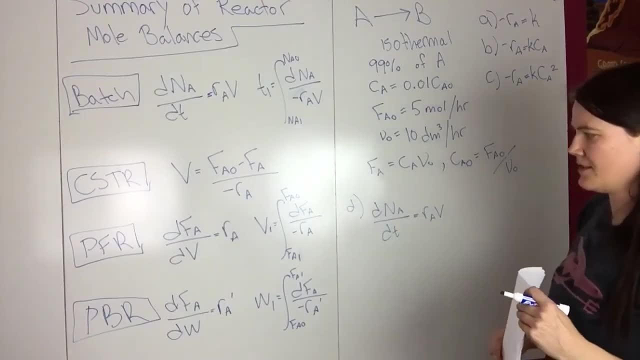 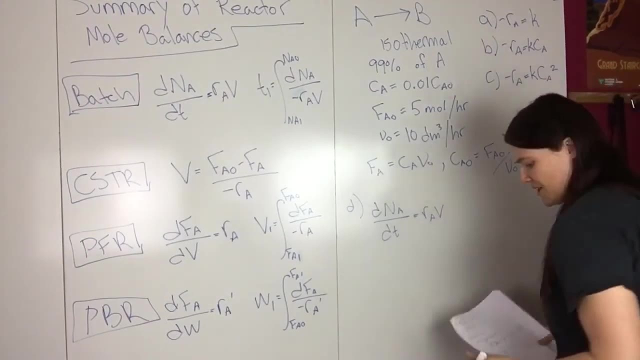 as the PFR in In A, B and C, So We want to Go ahead and rearrange this. First of all, we know that the volume is constant because it's a batch reactor and It gives you the volume. so 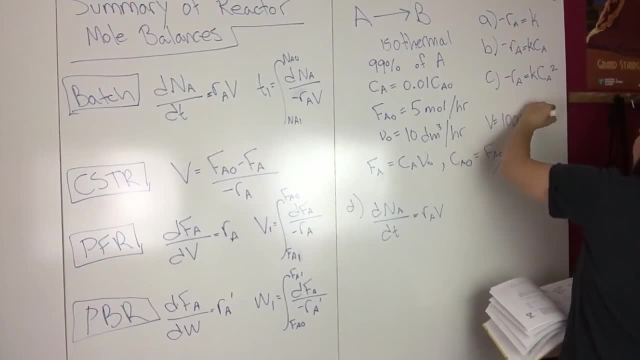 V equals 1000 DM cubed. Oh, and it also gives you C A naught for this one. So Because you, Because there's no flow, So for this, For part D, only C A naught. Well, actually that's the same as. 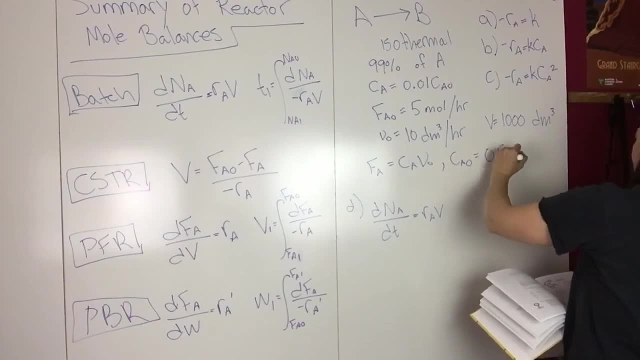 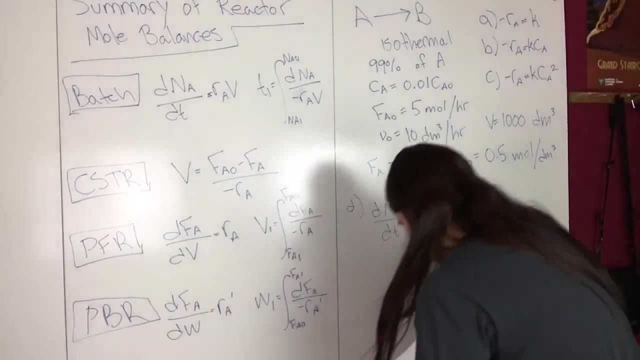 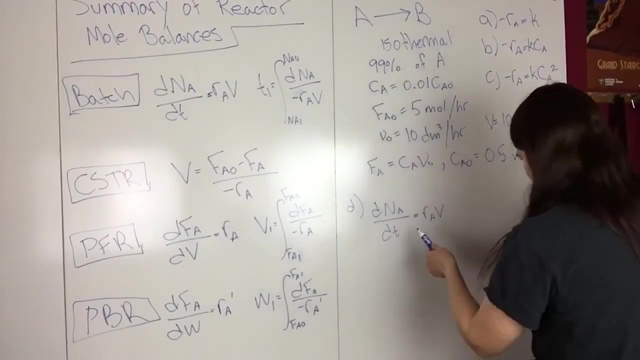 we calculated before, But it gives you that C A naught is 0.5 moles per DM cubed. Alright, so then We want, We want to solve for time. So let's go ahead and rearrange this, Or we could just start. 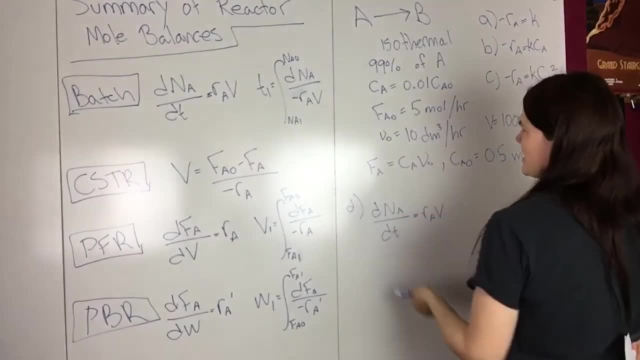 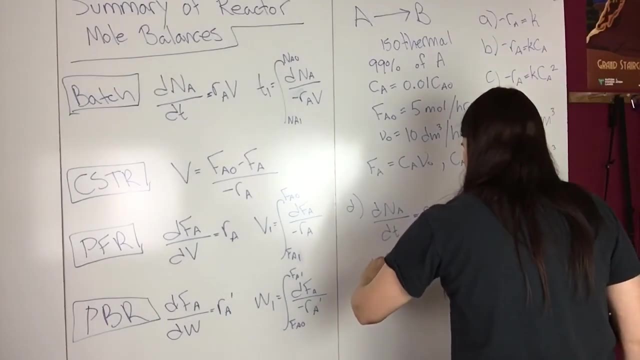 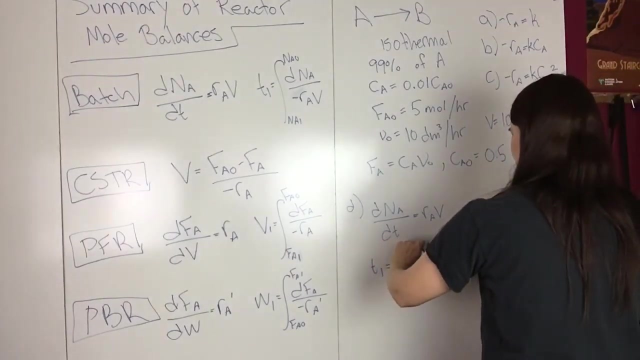 with that. We could just start with this equation. So I'm gonna, I'm gonna do that, I'm just gonna start with this one. So T equals N the moles at So, moles at time 1 to moles at time 0.. 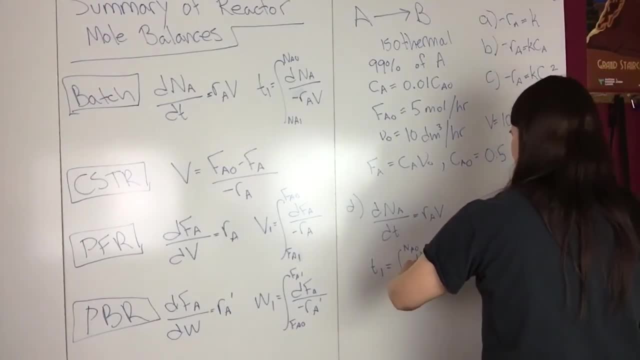 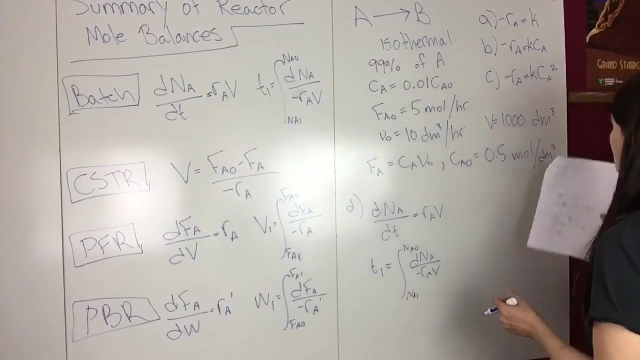 D and A over minus R A V. So then, plugging in the information we have. for the first one, we know that this R A is just K, so We have N A 1, N A naught. 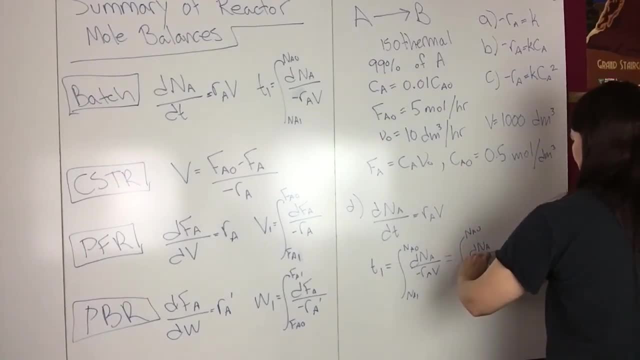 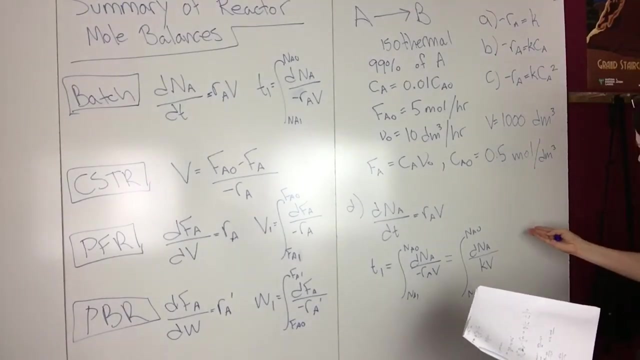 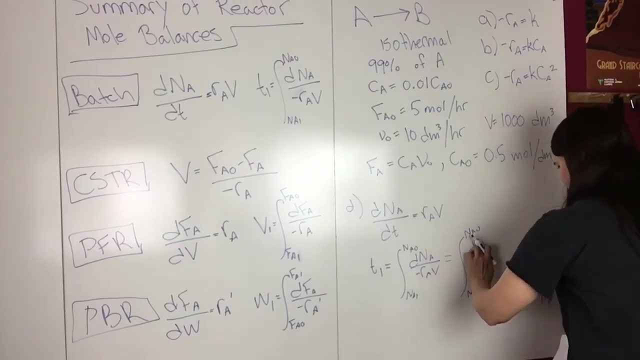 D, N, A, over K, V, and So then you can just integrate this and you know, You know all the information. So you know, Let's see. Yeah, you know, Actually change these to Plugging stuff in So you want to use concentration. 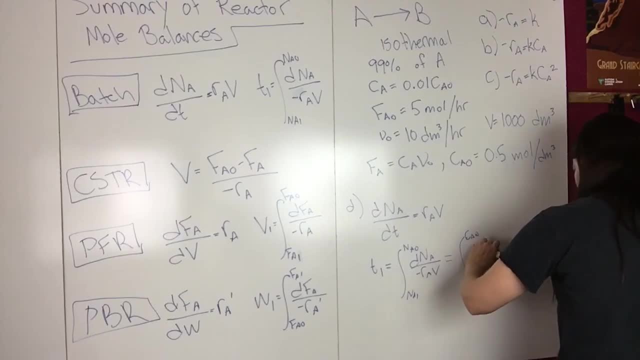 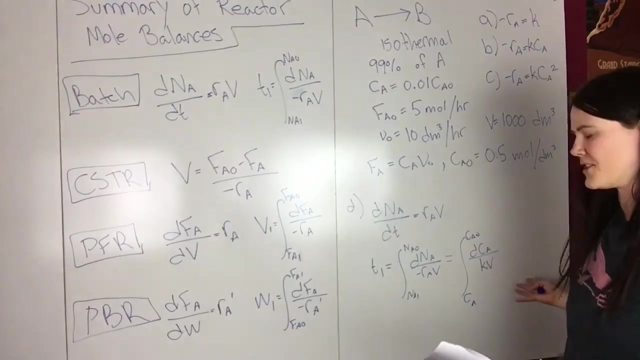 D, C A, Alright. So yeah, You know what K is, You know the volume, You know C A And you know C A naught, So you should be able to, Once you integrate this, you should just be able to. 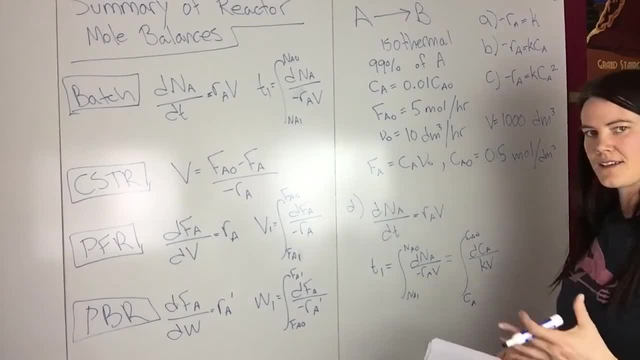 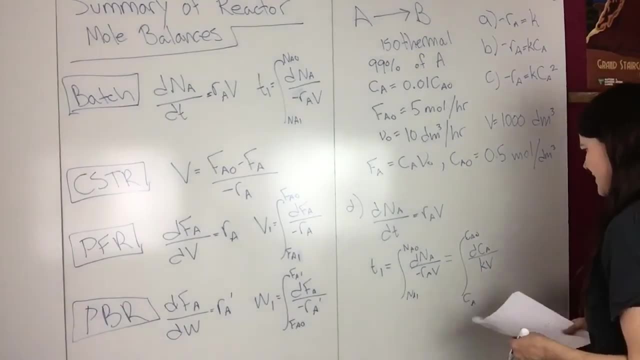 plug everything in and solve it, And then it's, And this is basically the same method as what I already did with the PFR. So, And you can do this with all of the problems or all of these, So D.